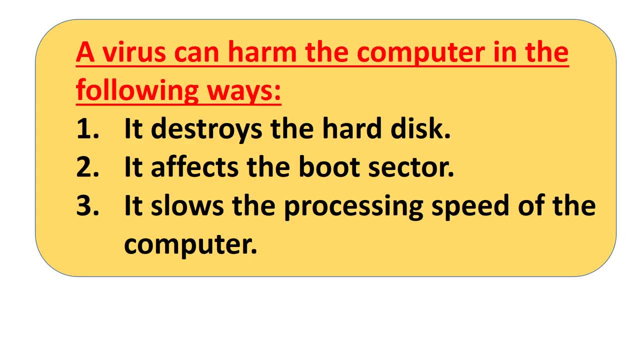 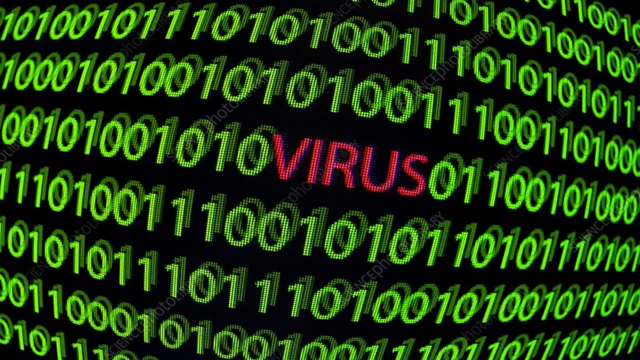 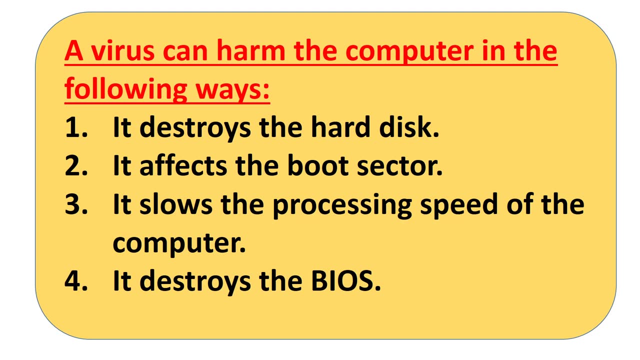 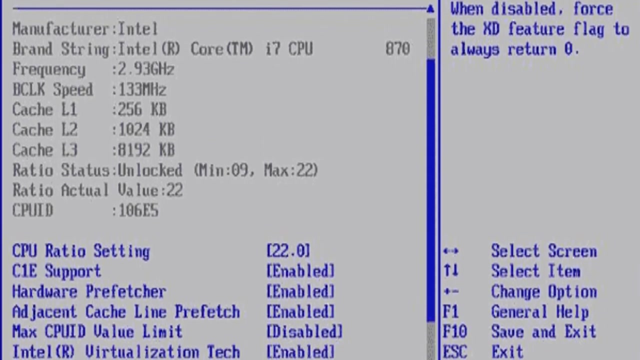 Third, it slows the processing speed of the computer. The computer viruses are automatically loaded into the main memory of the computer and remain in the memory. This slows down the processing speed of the computer. Fourth, it destroys the BIOS. This destroys the BIOS of the computer. This affects the startup process of the computer. 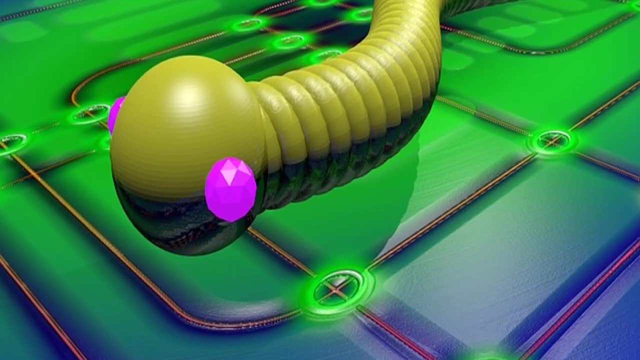 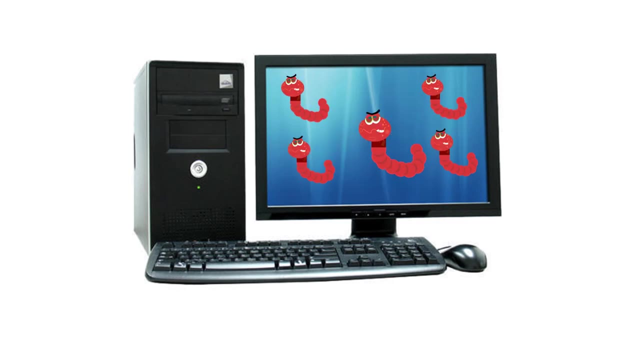 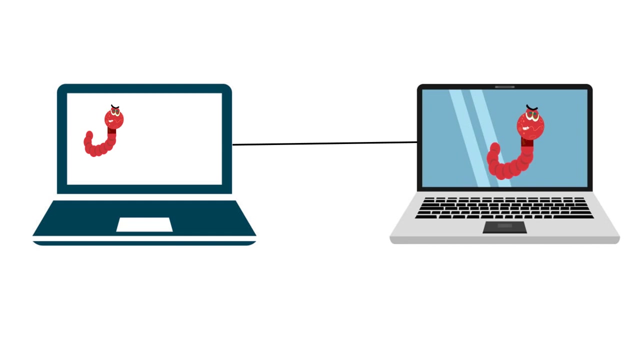 Worms. Worm is a self-replicating program and does not require a host program. The worm creates a copy of it and causes it to execute. No user interference is required. Worms are named for the way they move from computer to computer using networks. This action 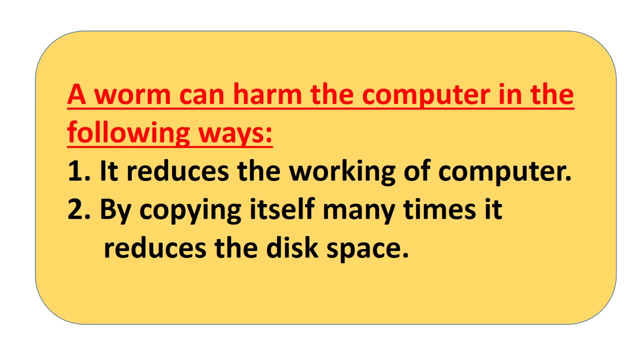 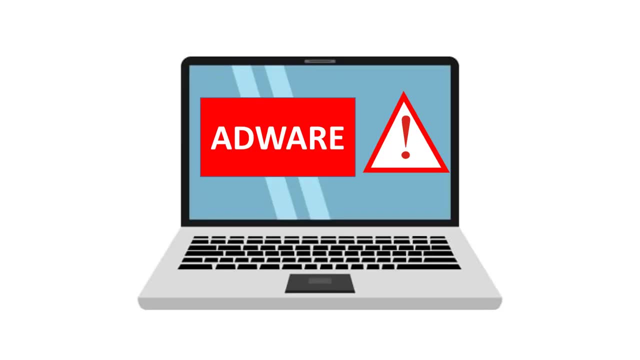 gives many worms a high speed in spreading themselves. A worm can harm the computer in the following ways: It reduces the working of computer By copying itself many times. it reduces the disk space Adware. Adware is an advertising supported software which automatically displays 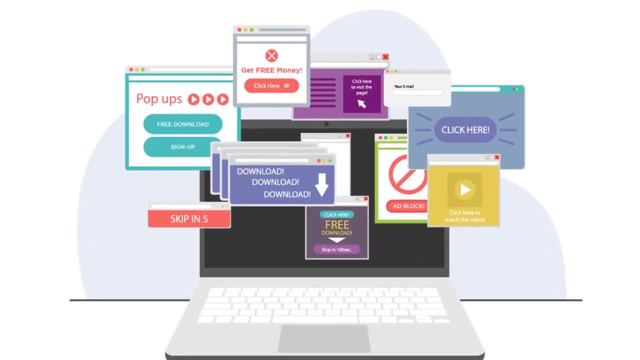 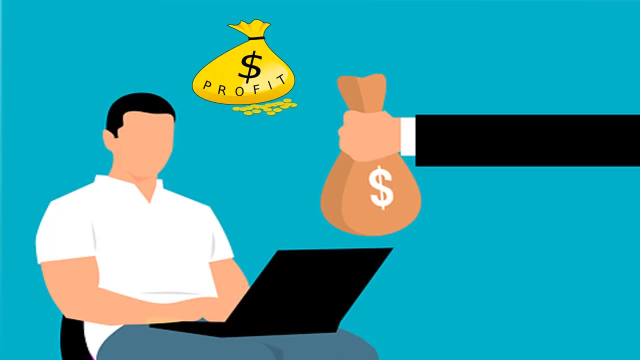 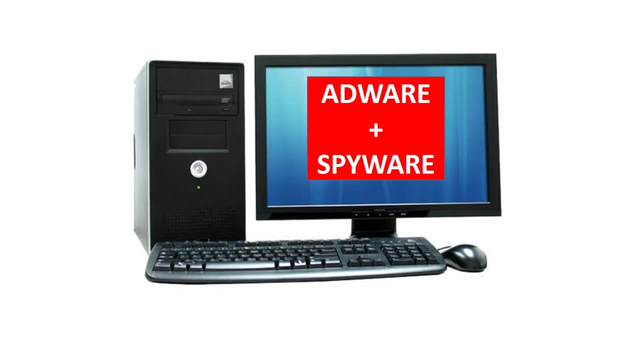 and downloads advertisements to a computer. when users are connected to the internet, These advertisements can be a pop-up. The objective of the adware is to generate revenue for its developer. Adware by itself is harmless, But some adware may also come with integrated spyware. 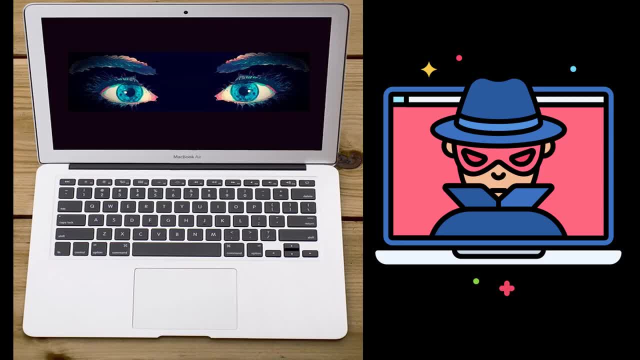 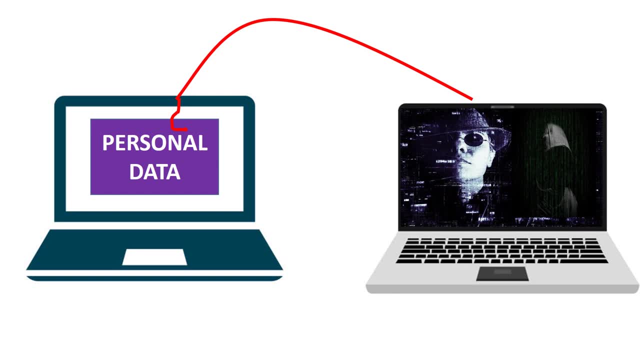 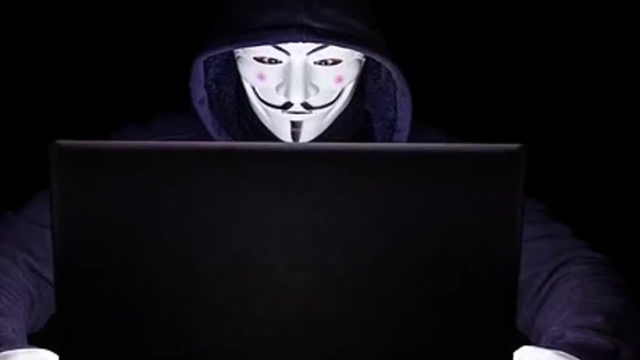 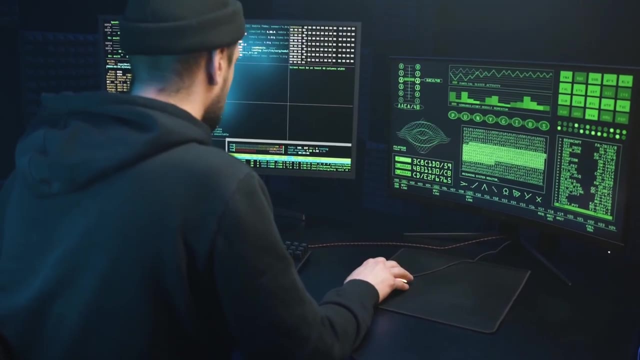 which can have negative impacts. A spyware is a software that gathers information about a particular user or organization without their knowledge. Hacker Hackers are programmers who use their expertise for malicious purpose. The term notorious hackers, sometimes called crackers, refer to those who break into computers without authorization. 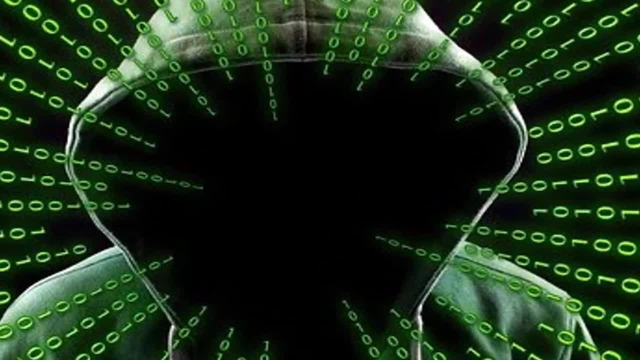 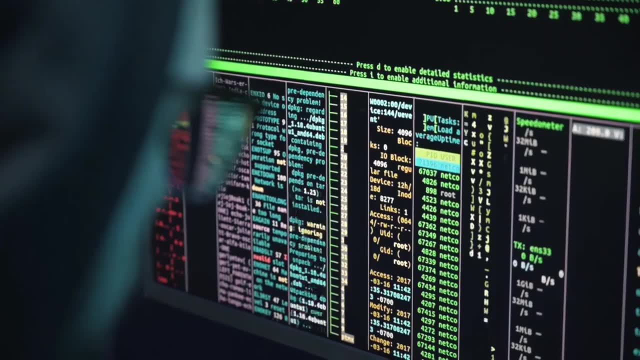 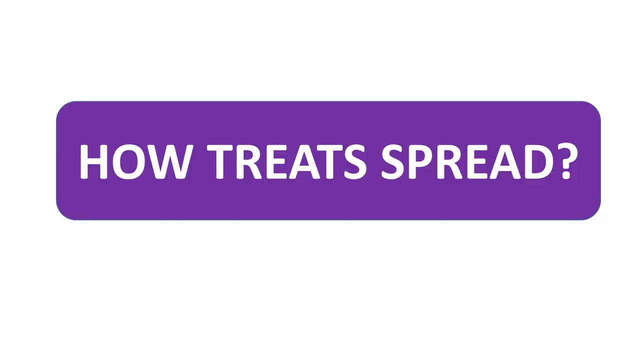 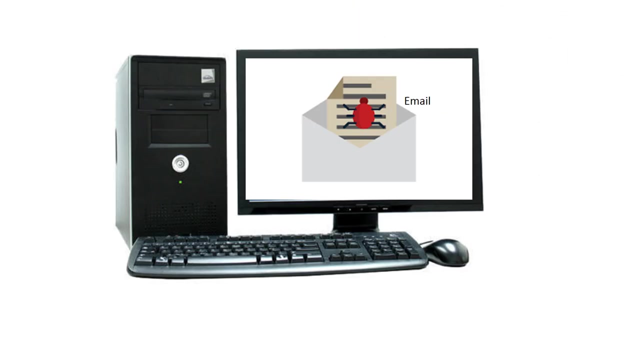 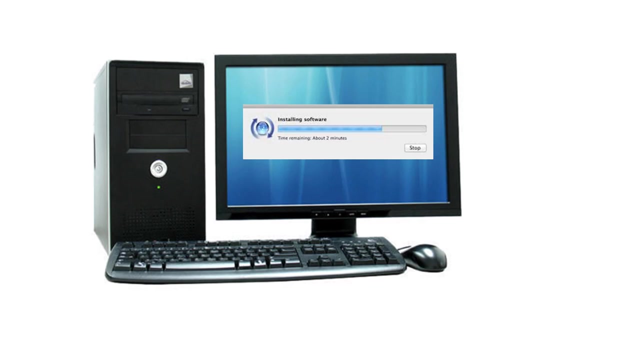 the hacking problem is widespread and serious. they get access to services without paying for them. they steal information for crime purposes. hacker gets unauthorized access to data and system and damages it. how threats like viruses, worms and adware are spread through infected flash drives or usbs, through email attachments, surfing insecure websites, installing pirated software. question time.